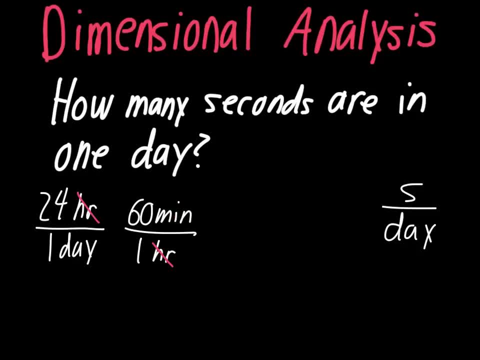 Remember, what goes up must come down. So now we need minutes in the denominator of the next one. So here we'd end up with 60 seconds in one minute. So again, since we end up with minutes on opposite sides, we can cross those out. 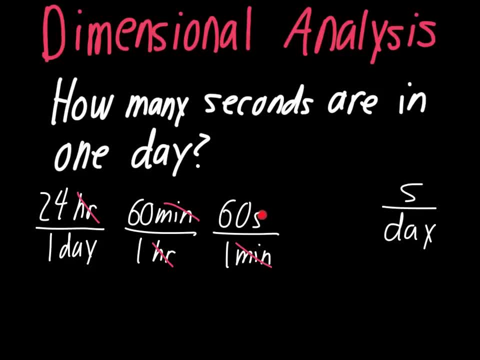 Now, if you look carefully, what we're left with are seconds in the numerator and days in the denominator. We wrote that one down in the very beginning. That's what we want. That's going to be the breakdown for our answer. So what you end up doing then? for this one, it's easy. 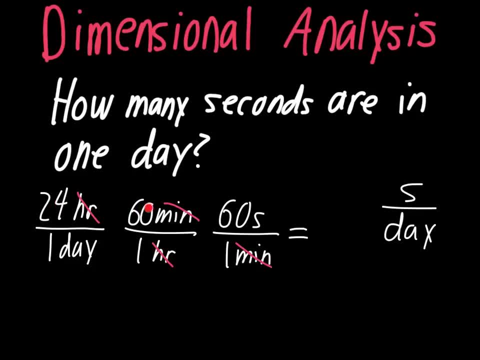 Since all of our numbers are in the numerator, you just multiply each of these together. If you had a number other than one down here, you would then have to multiply each of these together. multiply each of these together and then divide your top number by your bottom number. 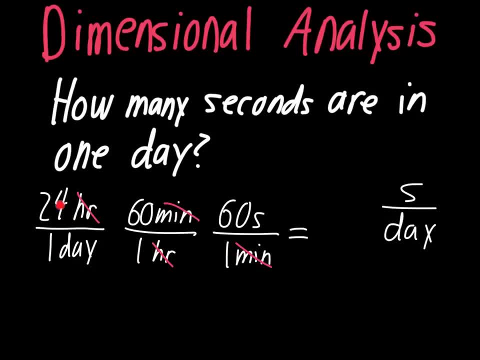 But since we have only ones in the bottom, all we have to do is multiply 24 times 60 times 60 again, which comes out to quite a few. We end up with 86,400 seconds per day. You can use dimensional analysis to break down any kind of problem like that. 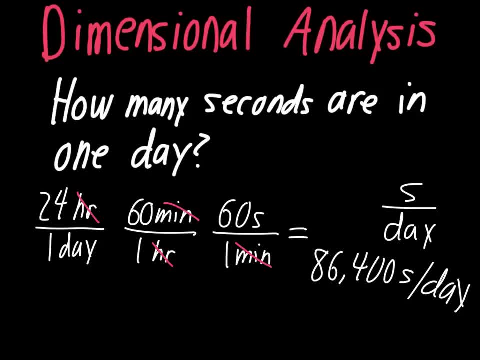 Again, the two important things to remember is, once you read the problem, you've got to figure out what the units are, that your answer is going to be in and then, if you just remember, what goes up must come down, What goes up must come down. 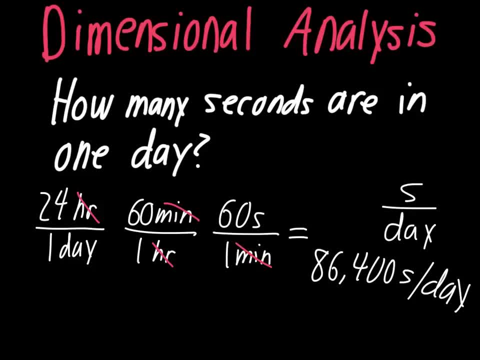 That's going to keep crossing. You're going to have to find out the appropriate units for you, and you'll eventually work your way to the answer to the problem. So we'll take a look at one for the next example that's a little bit more complex. 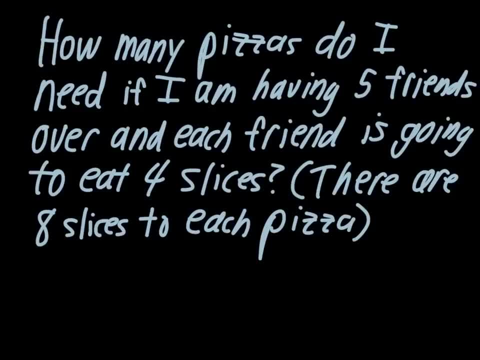 but maybe also a little bit more practical. So in this example you're trying to figure out how many pizzas you need if you're having five friends over, and each friend is going to eat four slices of pizza. So I added in an extra little piece of information for you. 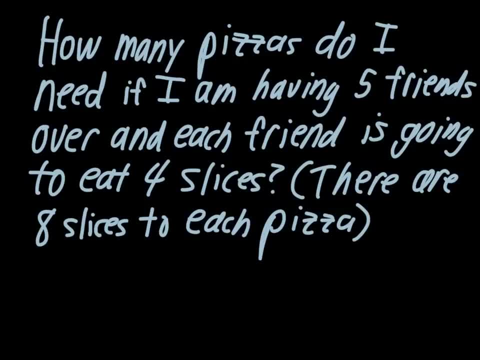 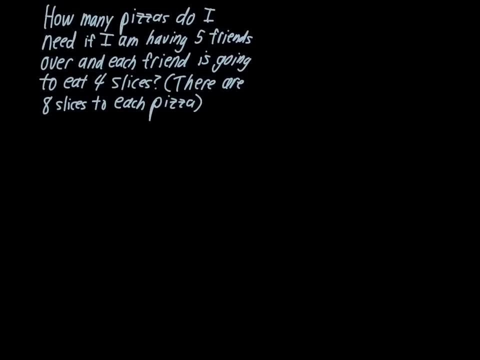 There's eight slices to each pizza. So to start off, I'm going to shrink this down just a little bit. We'll blow it up again if we need it, but sort of shrink that down and put it up in the corner to give us some room. 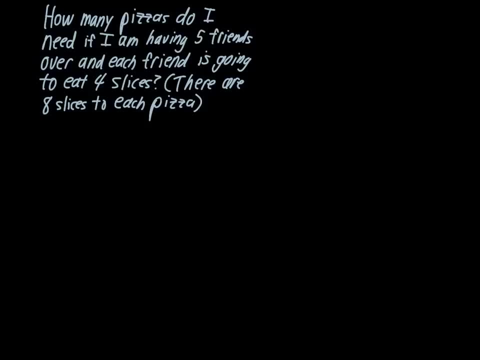 Like I said to you before, the first step is to figure out the units for your answers. So we're trying to figure out. you know, how many pizzas are we going to need? So that's going to be our answer To start off. we just have to go through and begin this problem. 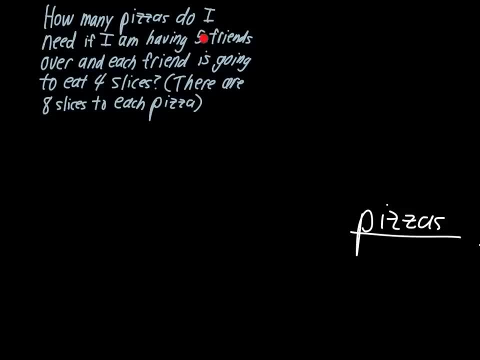 We said here in the beginning that we're going to have five friends over, So we'll start off with that, since that's the first piece of information in the problem. So we'll say: there's five people. Now. this is a good example of one where you don't always need something in the bottom. 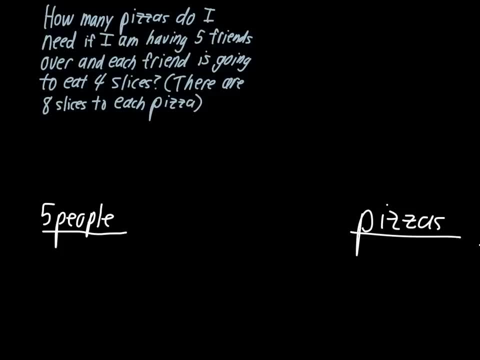 We're just going to leave the five people up there by themselves for now. The next step, the next piece of information that we have in the problem, is that each friend is going to eat four slices of pizza, So we'll put that one in. 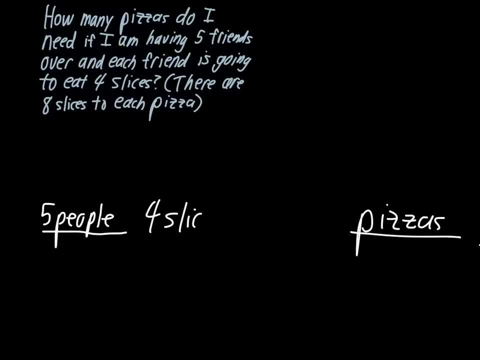 So we've got four slices for each person. So people and person- those cross out. I know it's not exactly the same word, but we've got- we're basically just going from like plural to singular right- Four slices for each person, five total people. 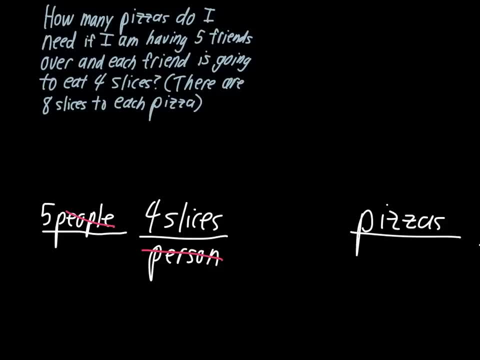 It's still the same kind of units, So we're crossing them out. That whole idea of what goes up must come down. Those two have to be opposites and they've got to cross off from one another. The next piece of information in the problem tells us there's eight slices to each pizza. 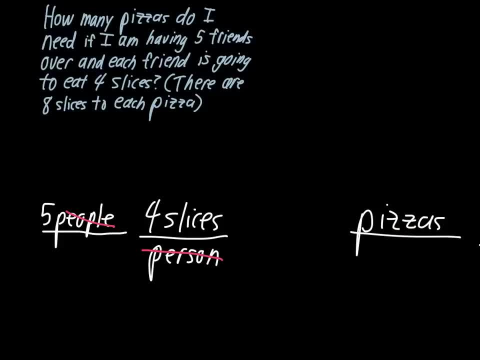 This is good. Pizza is the unit that we're trying to end with, So we'll put pizza on the top here, since we need to end with pizzas. One pizza has eight slices, So now, if you look, we can cross out slices. 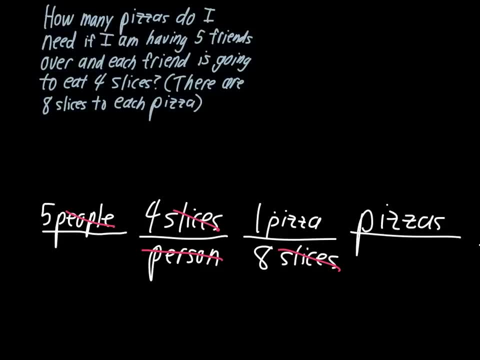 Now this problem becomes a little bit more complicated. If we're looking at this, we've got to go five times four, So that one ends up giving us 20.. I'm just going to write this up here at the top. And then we've got 20 divided by eight.